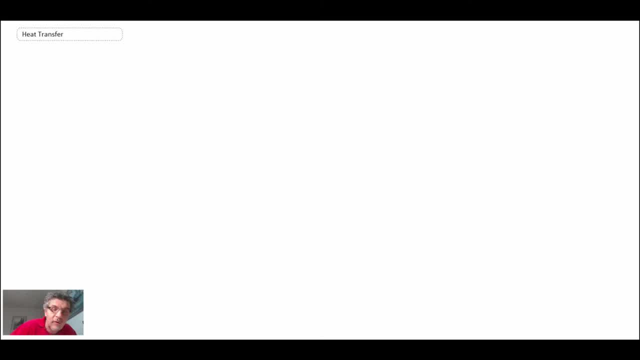 begin by looking at three different geometries, two horizontal and one vertical. So let me sketch those out and then we'll discuss them. So what we have here are three different geometries, two of them horizontal and one vertical, And these are the plates that are either heated or cooled, and I've indicated the temperature's blue. 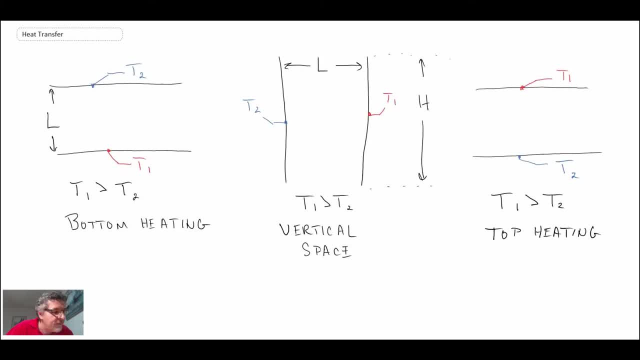 would be a cooler surface. red would be hotter and there is a fluid in the space between these two plates, be them horizontal or vertical. So let's begin and take a look at what is happening over here: bottom heating. Now, what is going to happen with bottom heating is the fluid adjacent to the wall. 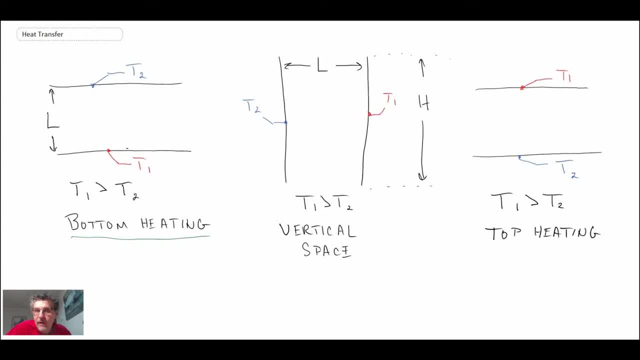 is going to heat up, and when it heats up it will become less dense and consequently becomes buoyant and it moves upwards. and so it'll move up like this, and when it gets up near the upper wall it starts to cool. and when it begins to cool it becomes more dense and consequently it then starts. 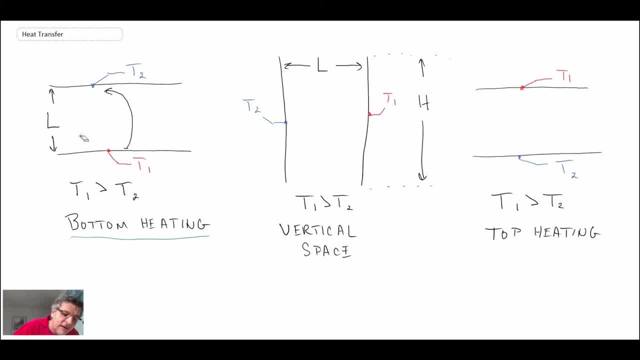 to descend, and what we then find? that's not a very good arrow. let me redo that. what we then find is we get these cells developing and we refer to those as being convective cells that exist within the enclosed space, and so that's what happens with bottom heating, and there's a certain 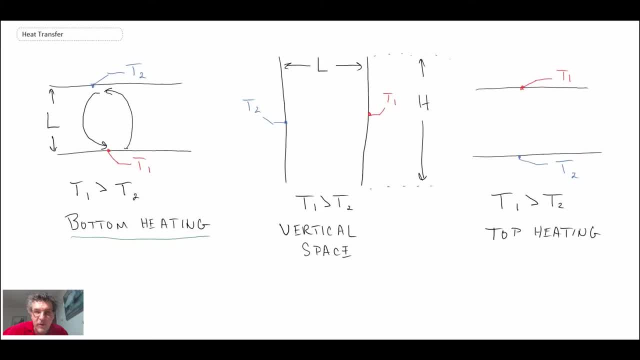 temperature differential before that begins to take place. Below it it won't take place and we'll be talking about that in the next segment. Now looking at vertical space, so this might be something like the cavity between windows or in the cavity of a wall, of a. 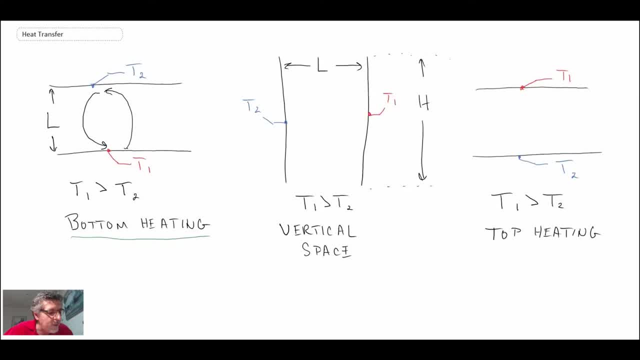 house where you have studs and then drywall and plywood on the outside. and what is happening? again, the fluid on the right hand side surface here is going to heat up and it's going to move, but we usually with a cavity, we're going to have some sort of confinement at the top and the bottom. 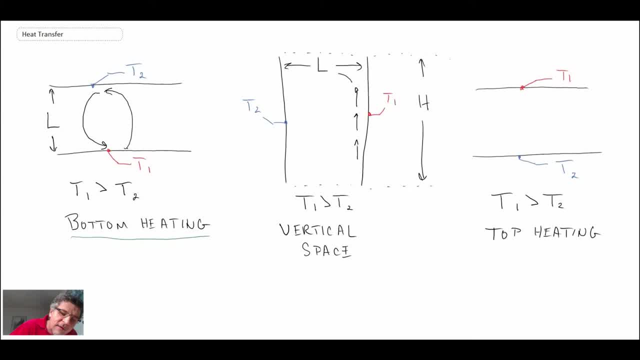 and consequently the fluid can't hit the top. it's going to have to start to come around and when it comes around it comes against this wall, which is now at a lower temperature, and it becomes more dense, and then it descends down to the bottom, but it can't hit. 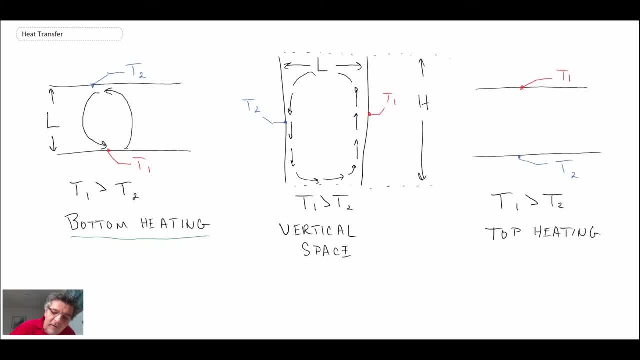 the bottom, it's got to turn again, and when it starts to turn, it starts to come back up, and that is the convective cell that develops within a vertical cavity. and then, finally, let's look at the last one here over on the right hand side, and here we have the case where the 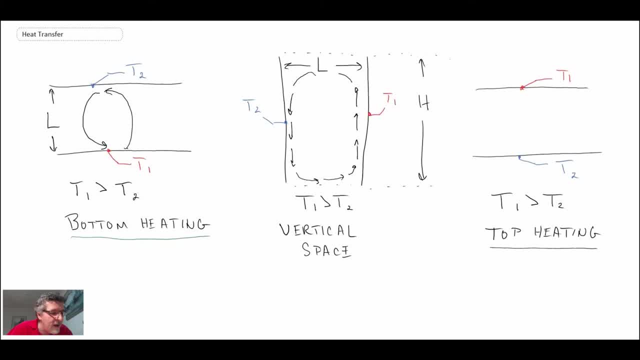 fluid plate is on the top and the cool plate is on the bottom, and this one, nothing exciting happens, it's just straight conduction, and that's because this is what we refer to as being stably stratified, and and so we go just from hot down to cool and that follows straight conduction going through. 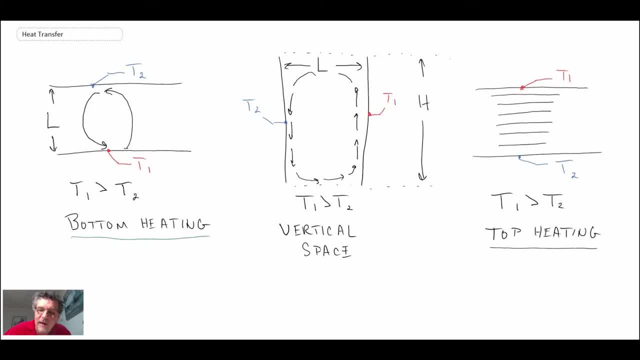 that. so the fluid does not go into motion when you have a stably stratified system like the one on the right. So with that, those are the three different geometries that we're going to be looking at in this lecture and when we're dealing with this. 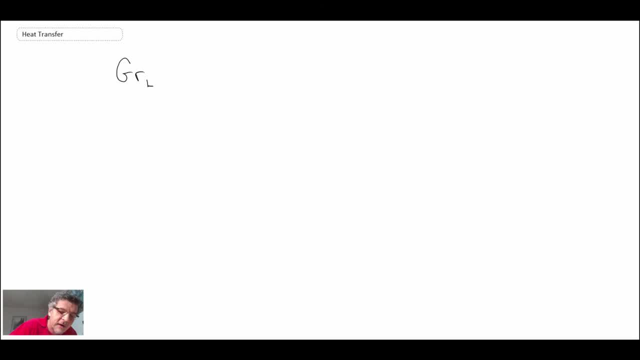 we have a Grashof number and the Grashof number with the characteristic length is l and l in all of those cases. hopefully I did that. no, I didn't put it here, let me put it there: l. sometimes you'll see delta, depending on the textbook. sometimes they'll use a, a delta there, but that can get. 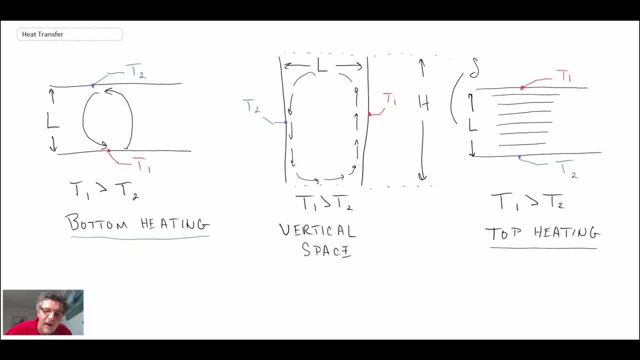 confusing, because that's what we said was the boundary layer thickness. so we're going to use the separation between the two plates and expressing that as a Grashof number, and then the temperature difference is going to be the hot surface minus the cooler surface, the length scale. 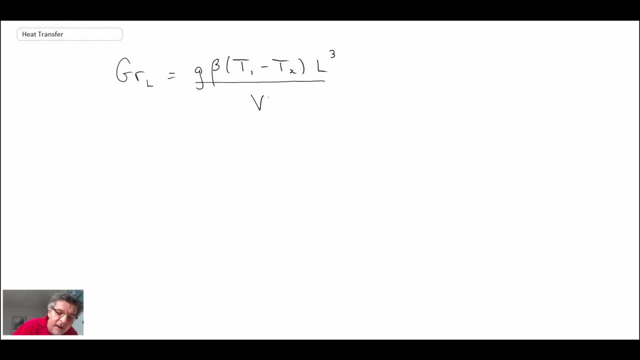 is l, and then we divide that by our kinematic viscosity, which is squared Neusault number. that is going to be evaluated again using l as the characteristic length scale, and then through this we have, through Fourier's law, the double prime would be watts per square meter. 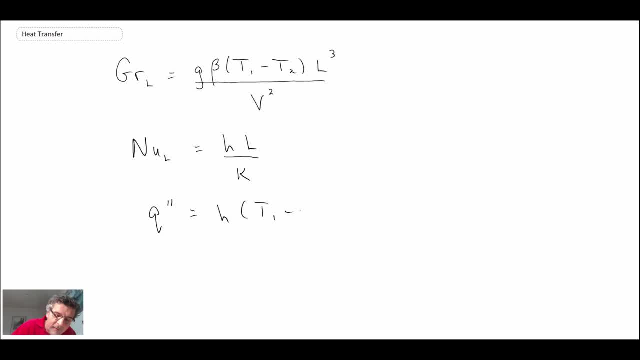 and then it would just be h times t1 minus t2.. So what we're going to be doing in this lecture is we're going to be finding ways, just like we've been doing with all the others, to estimate h, and we'll do that using Grashof number, Rayleigh number, Nusselt number, things like that. So 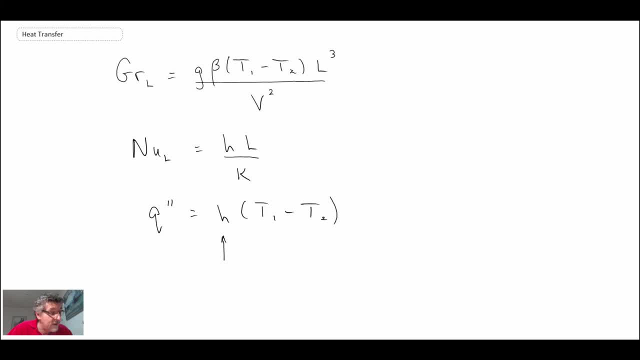 that is, free convection in enclosed spaces. What we'll be doing in the next segment is we'll begin with the horizontal, where we either have bottom heating or top heating, and we'll take a look at that flow field.